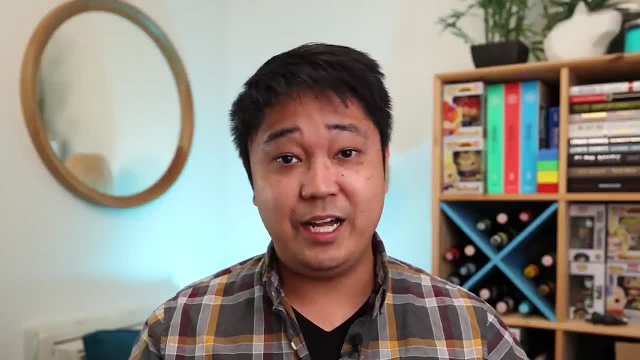 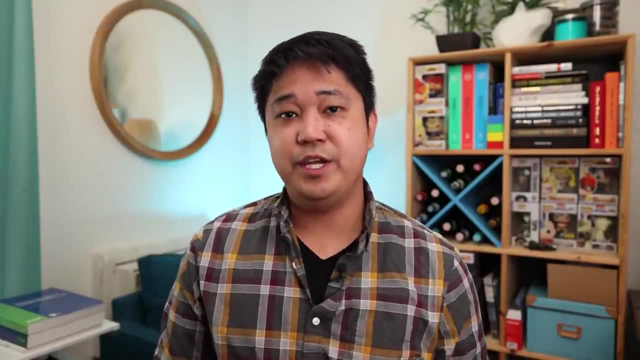 principals and the people in charge and see if they needed one. And that's how I got that internship. And even during those internships, even though I wasn't getting the engineering skills that I wanted, i still made the most of it. i learned how the public sector worked. i learned how the private 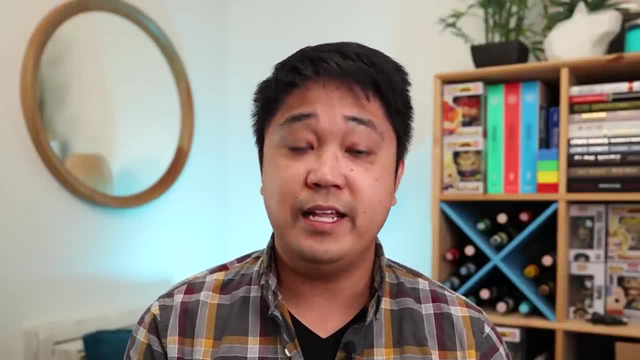 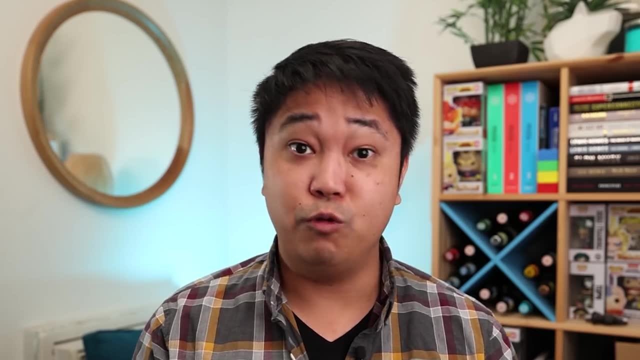 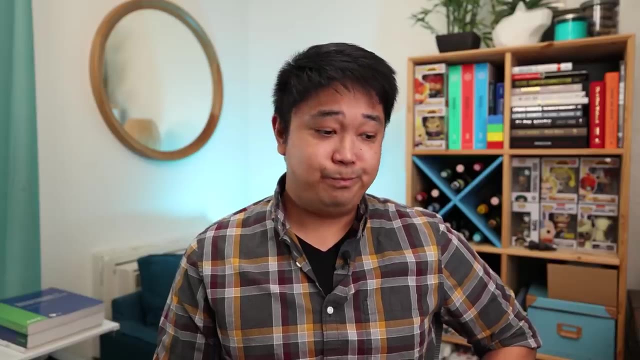 sector worked. i talked to the engineers and asked them what the engineering industry is like, what they do on a daily basis, and if they had any advice for an intern like me. you are responsible for your own education. 2014: this is when i was in grad school at uc san diego and um the first. 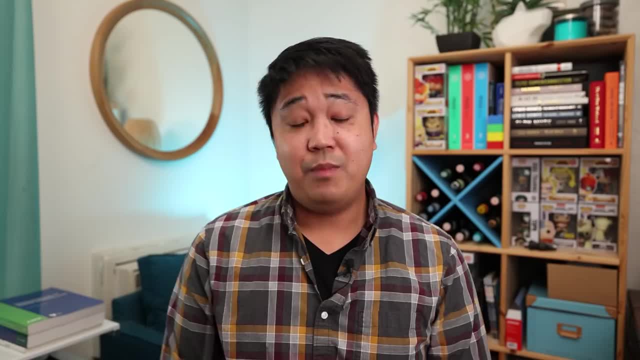 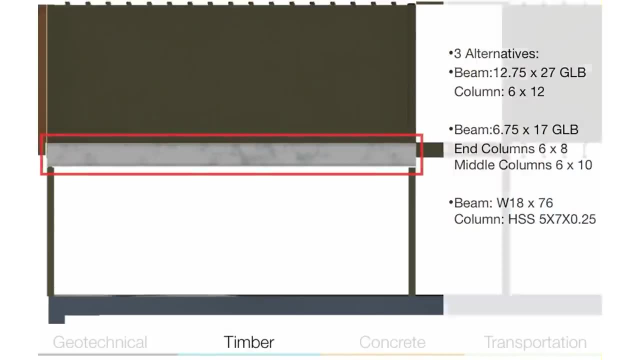 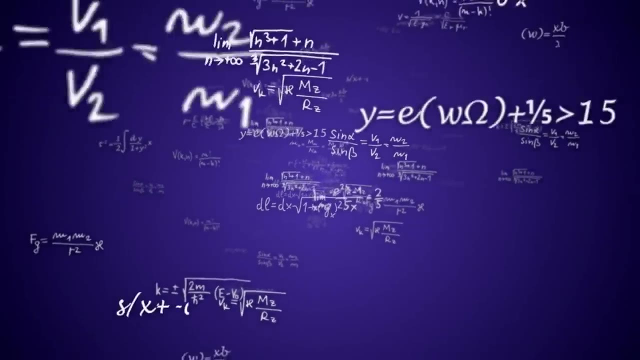 quarter at ucsd kicked my ass. my undergrad was at cal poly- one of words: a more practical school. we deal a lot more with the building codes and practical problems versus a uc system where it is a lot more theoretical, less design work, more of the theory, equations and math. oh man, so much math. 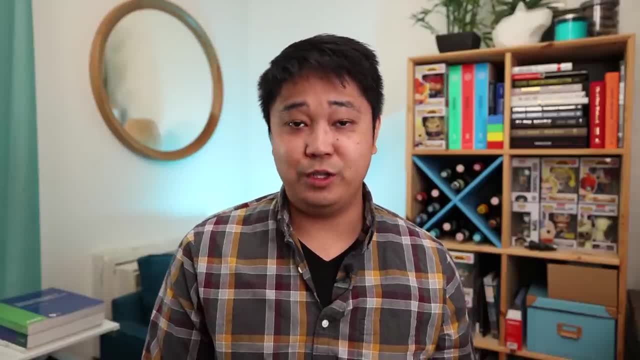 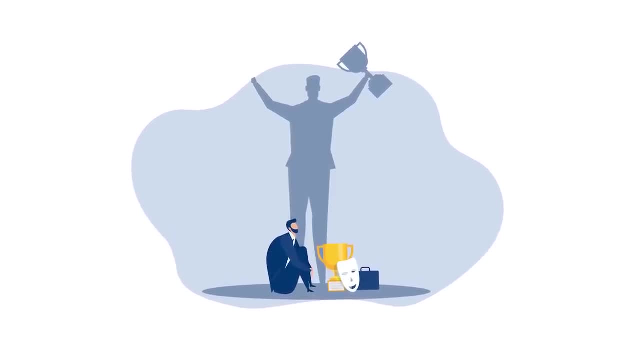 so much so that it was a shell shock for me. i was really struggling just to keep up with all of the math equations. in my first quarter i definitely had imposter syndrome. my gpa wasn't that great and, compared to the rest of my classmates and how they were doing, i was definitely not the smartest. 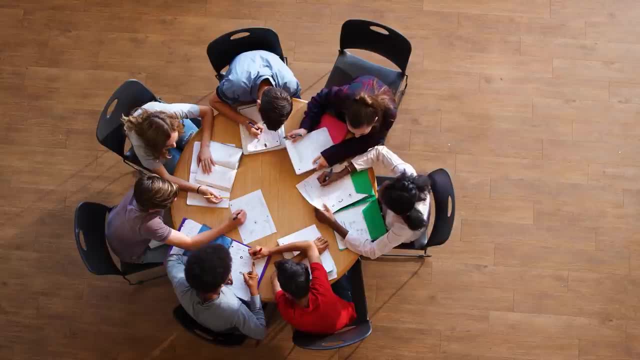 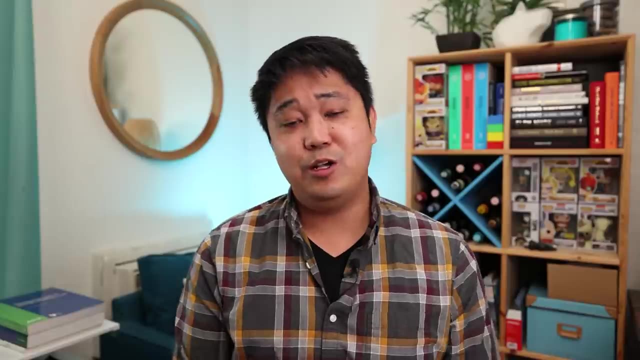 starting out in that first quarter. but it wasn't until i got into some study groups asked for help, went to office hours where i really started to improve and catch up with the rest of my classmates. this was also the year i got my first real structural engineering internship where i 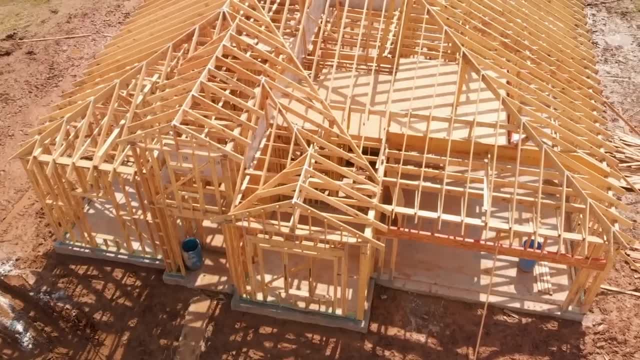 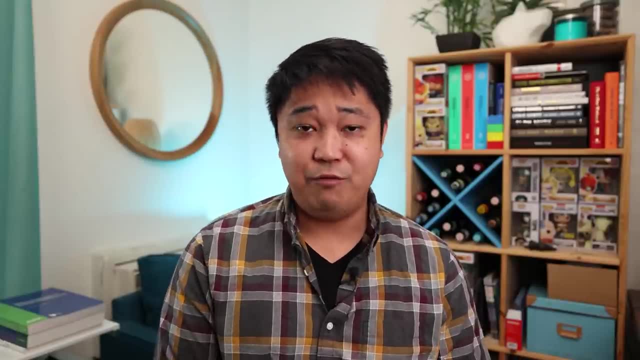 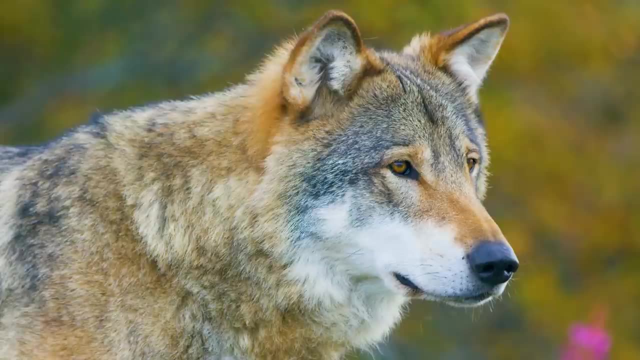 actually got to do the stuff i wanted to do: designing buildings, designing structural members, talking to other engineers that were in the company, that were from all different types of firms, and i learned a lot from them. lesson learned: don't be a lone wolf. know when you need to ask for help. know when you're stuck, because lone wolves don't survive and there's 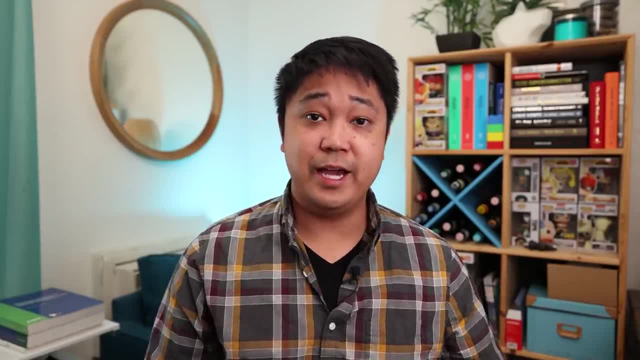 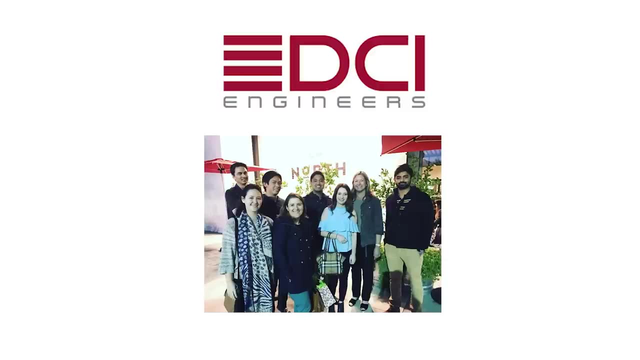 nothing wrong asking for help when you gave it a good shot and you need some guidance. 2015.. this is the year i started my structural engineering career at dci engineers. this was the year where i started to work on a lot of structural engineering calculations, learning a lot about 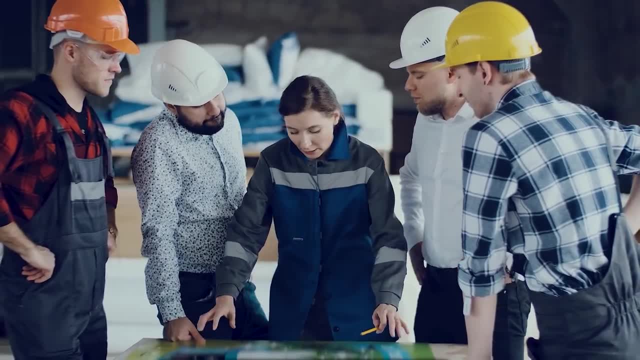 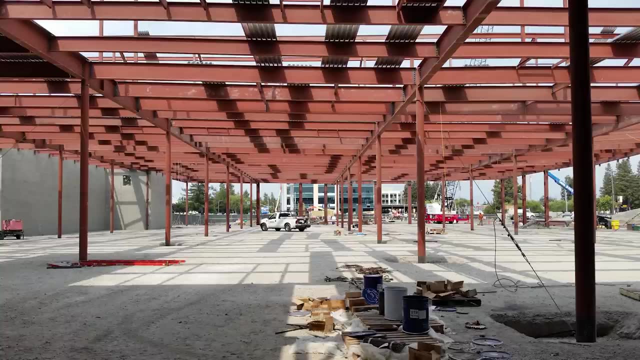 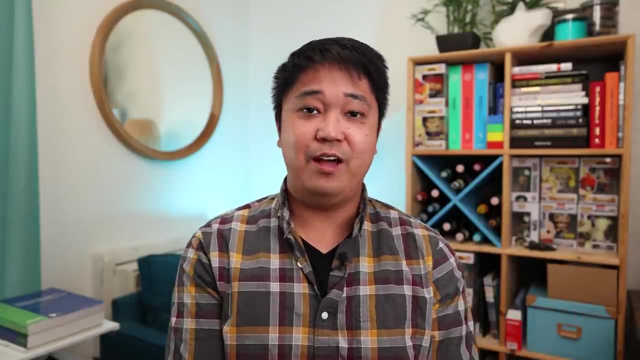 structural engineering drawings, how we work with architects, how we work with the contractors. and this was the year where i got to see some of my designs and construction discussions and eventually, full buildings getting built. i actually went to the site and i got to see them be built out into the field and just knowing the scale that went into it all. 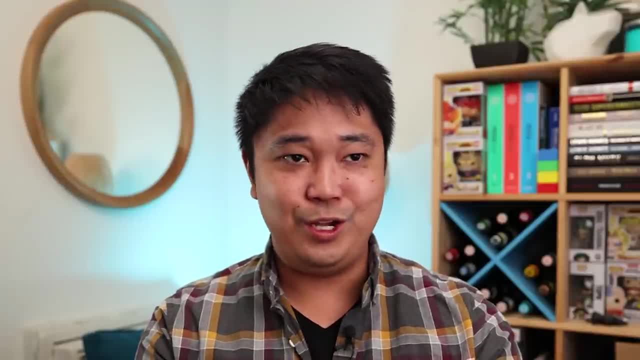 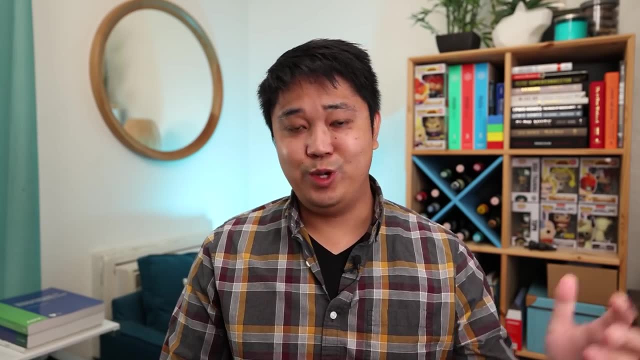 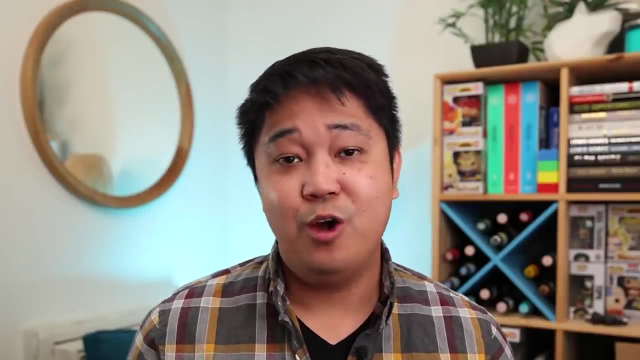 the work and effort that we put in, that was so fulfilling, and that's when i knew that this is the profession for me. lesson learned: you don't know anything when you start working in the structural engineering field, even with undergrad, even with grad school. there is so much you don't know and you will learn while you're at work. so ask questions. 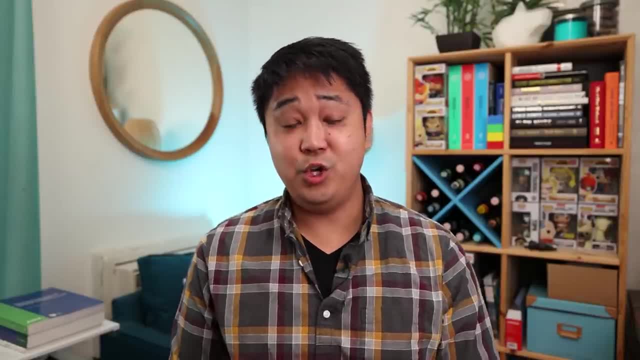 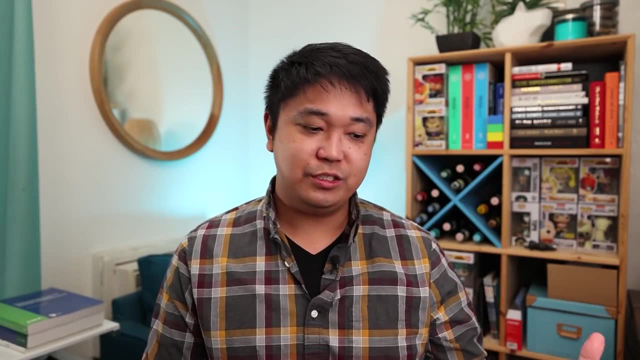 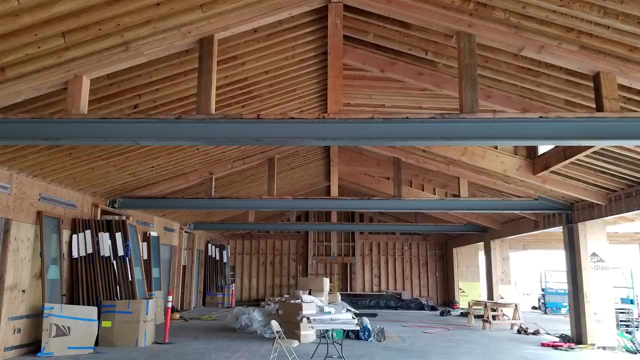 a lot of questions. they're expected if you're new and you're an intern. 2016: this was the year I got my PE license. I became a professional licensed civil engineer. this was also the year I got really good with wood from multi-story apartment buildings, custom clubhouses, custom trusses. I was learning a lot and 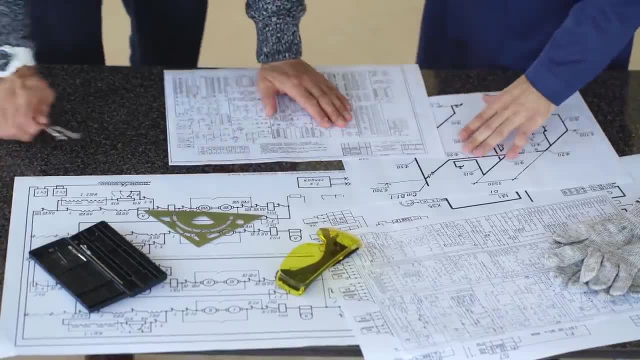 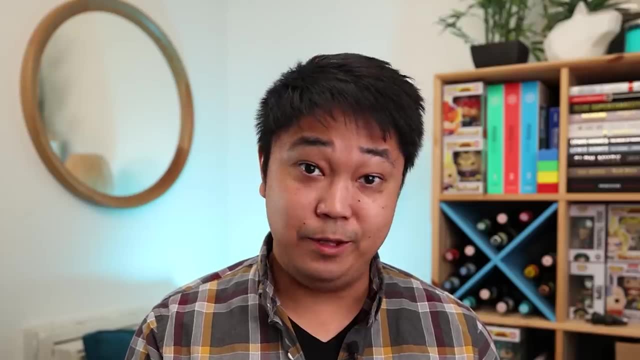 this is the year I also ran into my first tough plan checkers. designing and calculating out the structural systems of a building is great, but if you can't get it past the city, it's not getting built and you're usually dealing with a single plan checker. and if you get a tough one where they're questioning 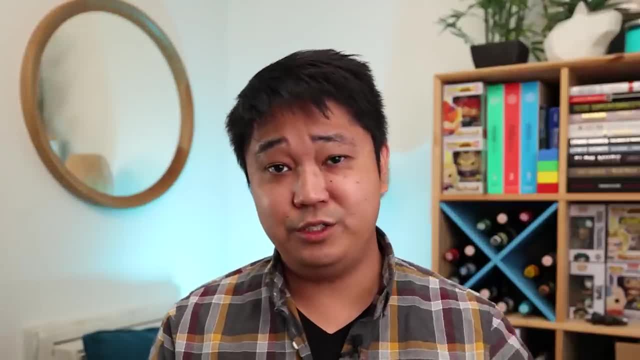 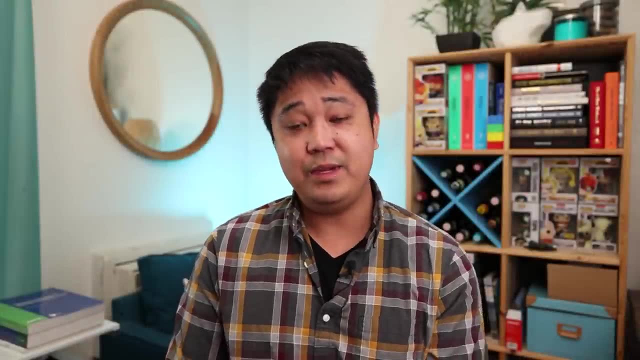 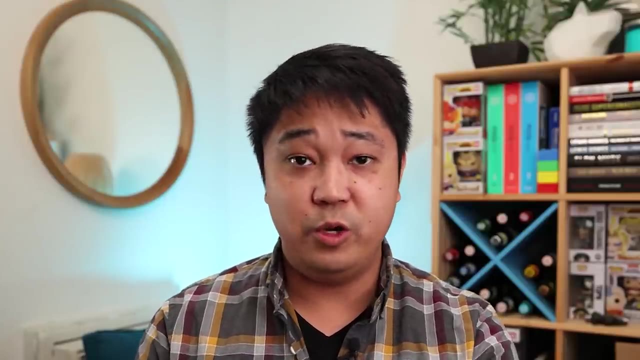 every little thing about your design. it can get rough, especially if the building has tight deadlines. lesson learned: being technically right isn't everything. you have to be effective, and that means you have to communicate your complex designs, thoughts and ideas to the plan checker or to the client, or to the owner and you. 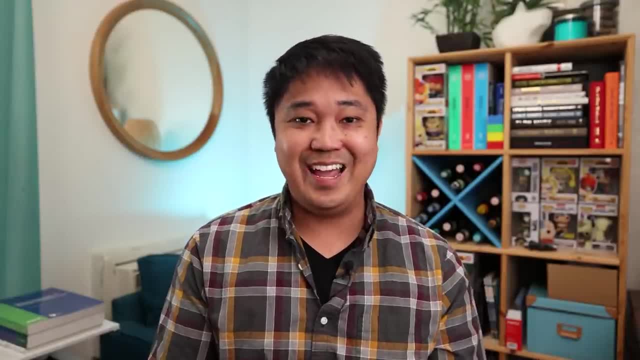 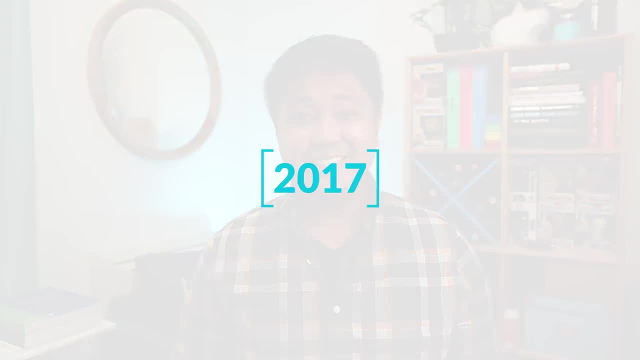 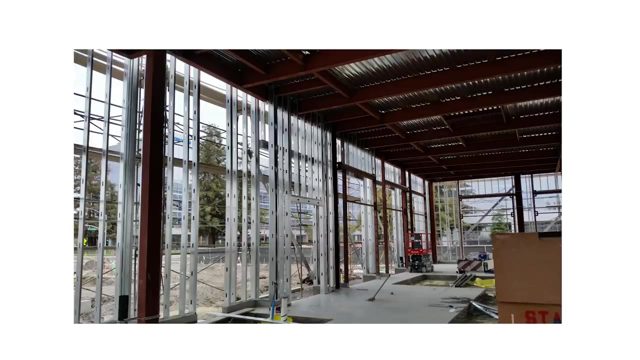 have to explain it in a language that they can understand. you can't just throw out all this structural engineering jargon, or else they're not gonna approve it and all of your calcs are for nothing. 2017: even more new projects: tenant improvement projects, cold-form steel projects, steel mowing frames, steel brace. 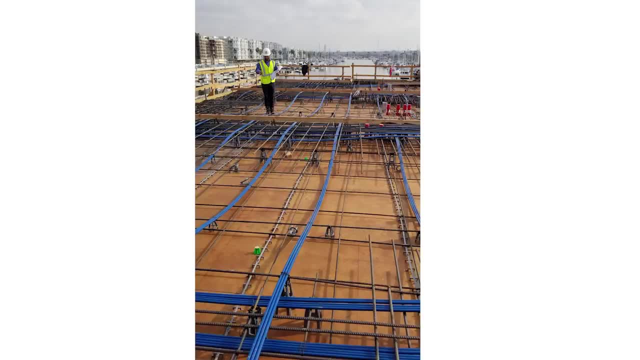 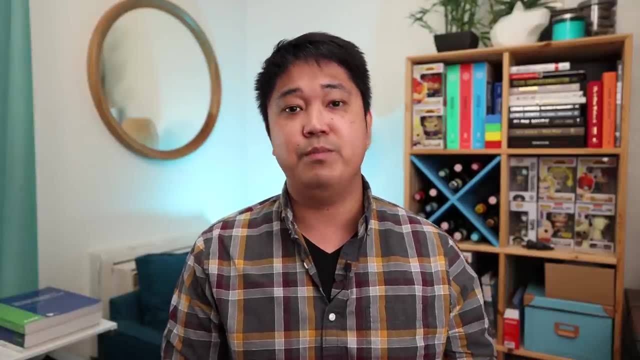 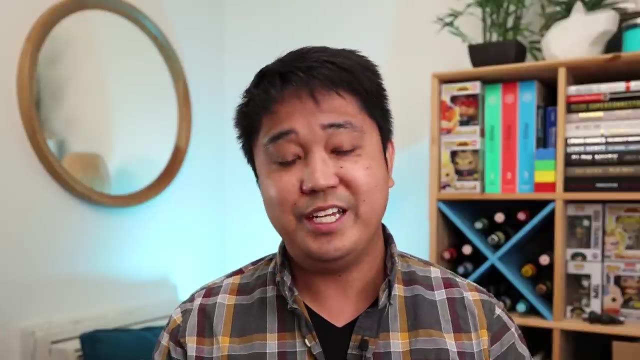 frames, open web, steel joists, post-tensioned concrete slabs and even high-rises. this was the year I got to learn a lot about different building materials and different building types. lesson learned: there is so much to learn in the structural engineering industry. a couple years in it, I'm just beginning to see how much of the things 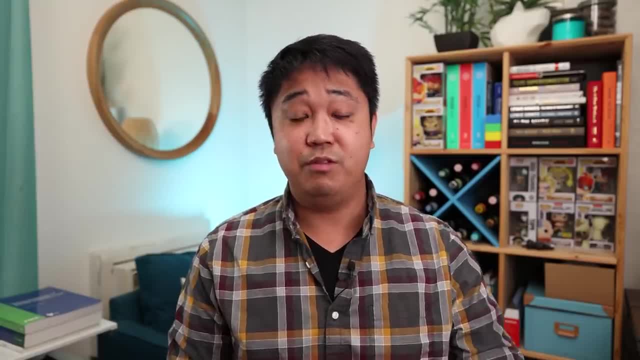 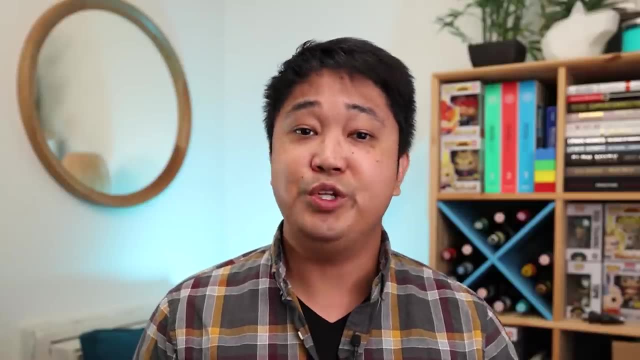 that I don't know about it. from all the different structural systems, from all the different lateral systems, different building types, there's just so much to learn, and I love that about the industry, because I'm learning something new every single day and if you're like me and you love learning new things, I highly 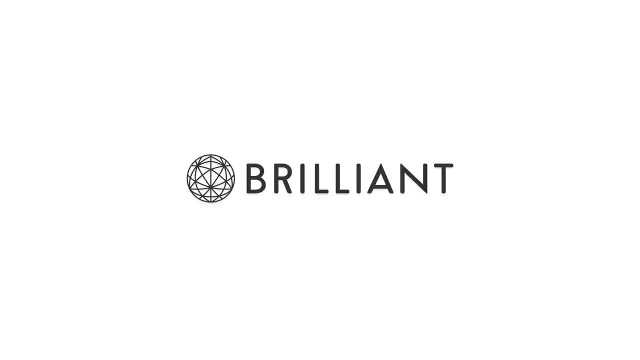 encourage you to check out brilliant, who I'd like to thank for sponsoring this video, brilliantisabrcom. Brilliant is an interactive STEM learning platform that helps you learn concepts by visualizing them and interacting with them And, as you saw from my previous years in university, I'm a very hands-on learner and I learn the 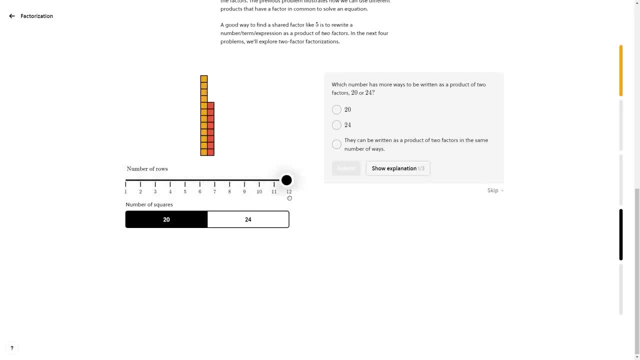 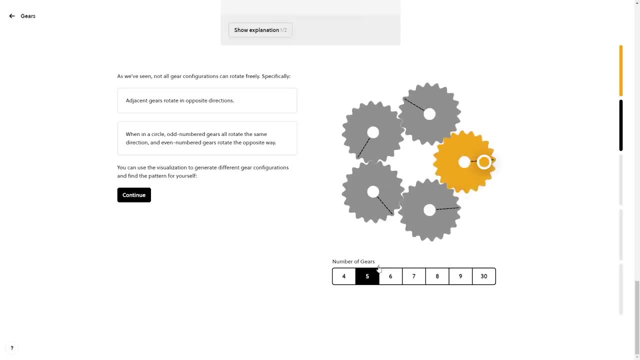 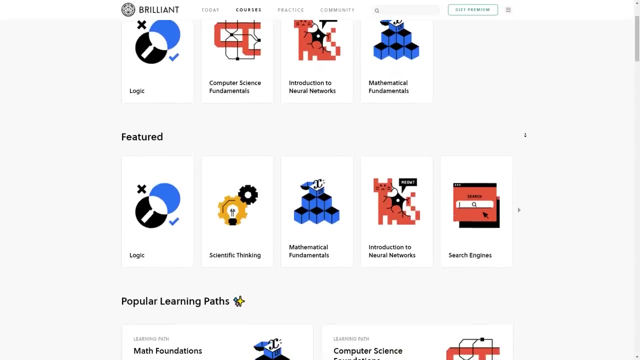 best by doing. Brilliant has and continues to add more interactivity to their courses, such as their scientific thinking course, where you'll dispense of the number crunching and mathematics in search of something more useful physical insight. They have a lot of other interactive STEM courses as well, such as computer science. 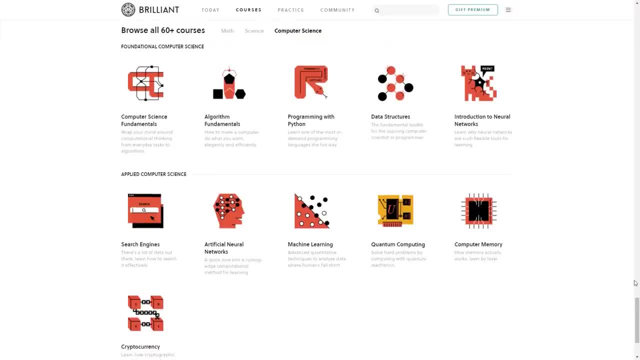 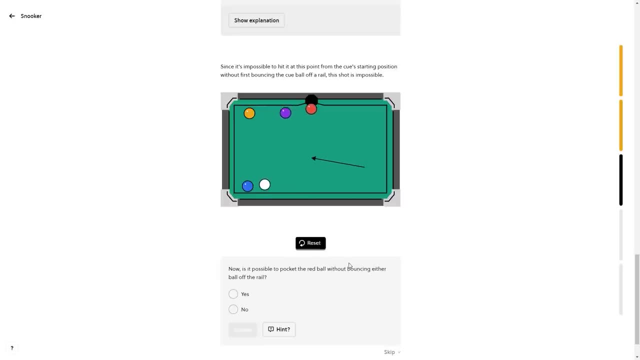 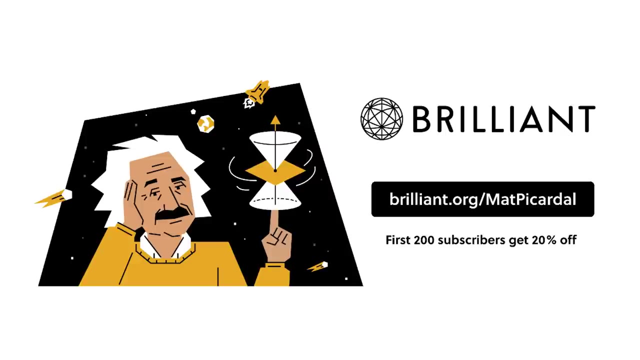 and programming, which can be very useful to know in the ever-evolving civil structural engineering industry. If you'd like to try out Brilliant for free and get 20% off a year of STEM learning, click the link in the description down below or visit brilliantorg slash Matt Picardal. 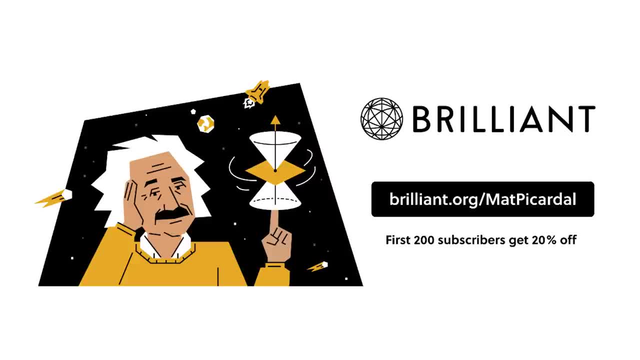 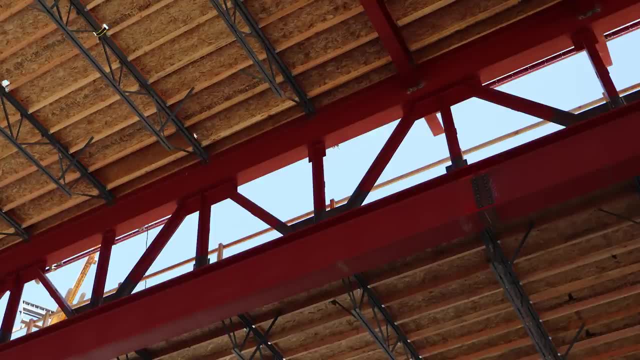 And note that this offer is only available for the first 200 people: 2018.. This is the year I got to work on custom long spans Design steel trusses, open web steel joists, complex diaphragms, buckling, restrained brace. 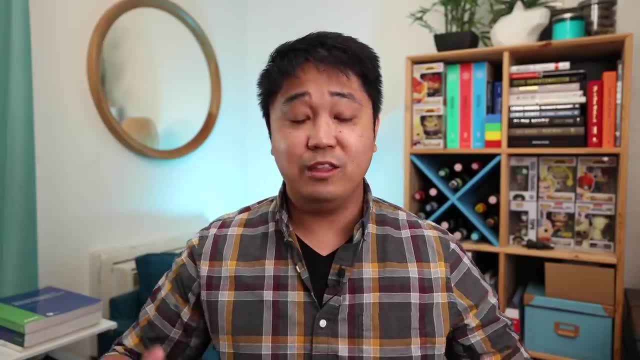 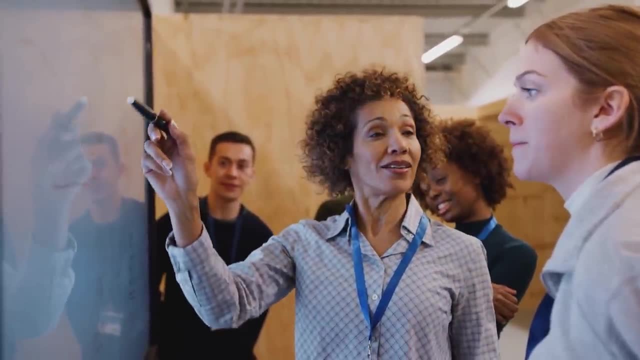 frames and foundation piles. This is also the year where I learned a lot about the value of mentorship in the structural engineering industry. I saw how fortunate I was to have the mentors that I had and seeing how much they've helped me throughout my career. 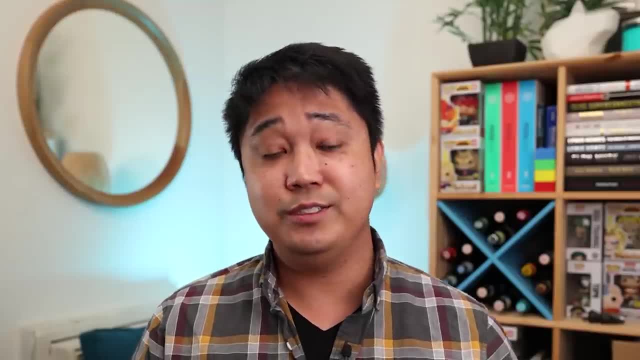 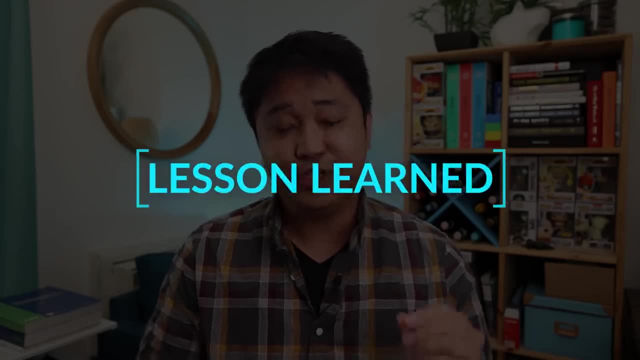 And as I networked throughout the structural engineering industry, I noticed that, you know, that is not something that all structural engineers have, And I saw how fortunate I was to have that Lesson learned. Learning is easy, but people skills are hard. 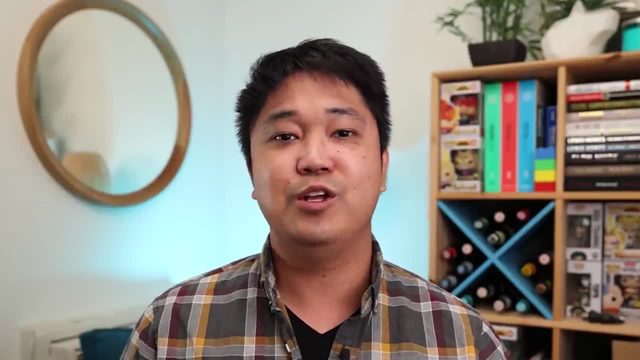 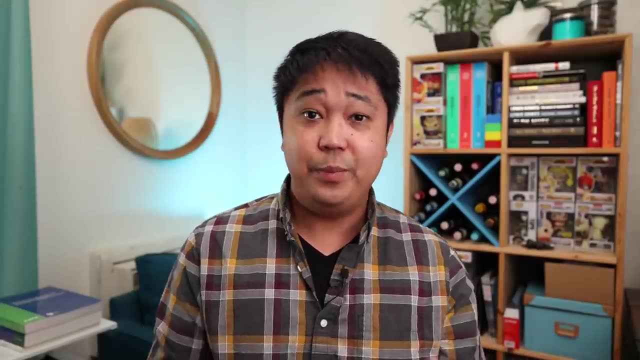 Year after year I would get thrown new engineering projects, new things to learn, and I had a good way of learning in those things. But people skills, especially for the typical engineer and for me, were a lot harder to learn but are so important in the industry. 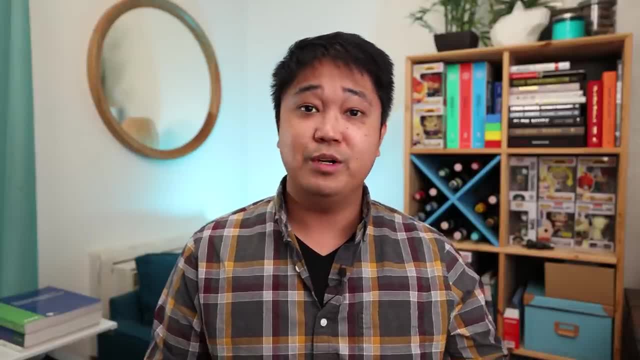 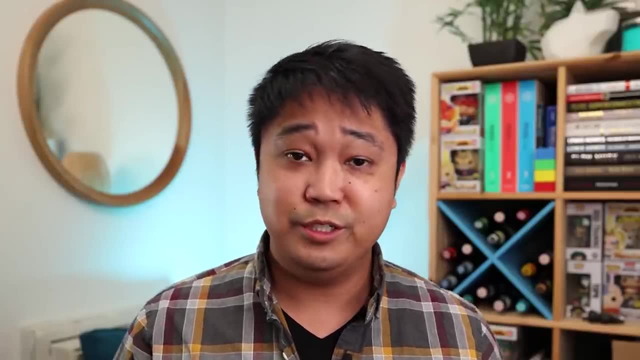 So I just started to learn more about leadership skills and people skills by reading books, watching YouTube videos, surrounding myself with good leaders and seeing how they work, and hopefully use that knowledge to help structural engineers live more fulfilling careers 2019.. I became a project manager. 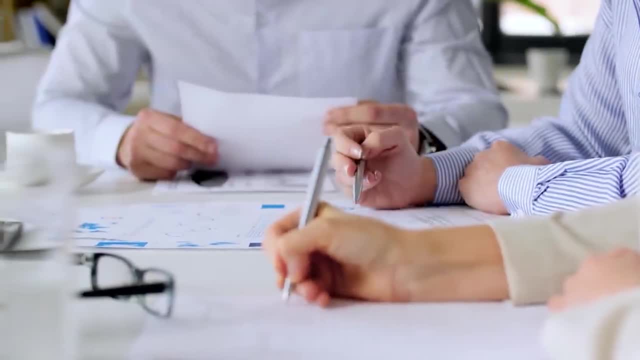 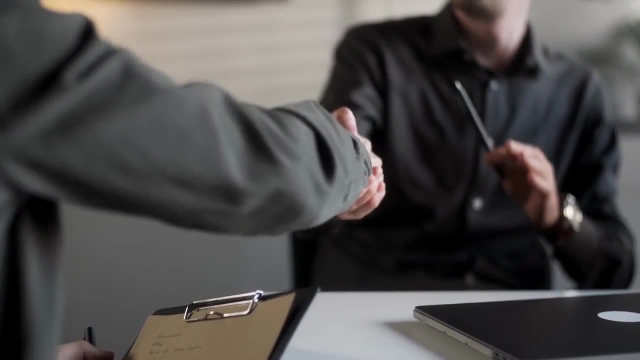 I began to work a lot more with the clients, seeing the bigger picture things of the project, billing, invoicing, writing and sending proposals out, winning work and making sure that current projects stay on schedule and on budget. This was also the year I got more involved in the structural engineering industry. 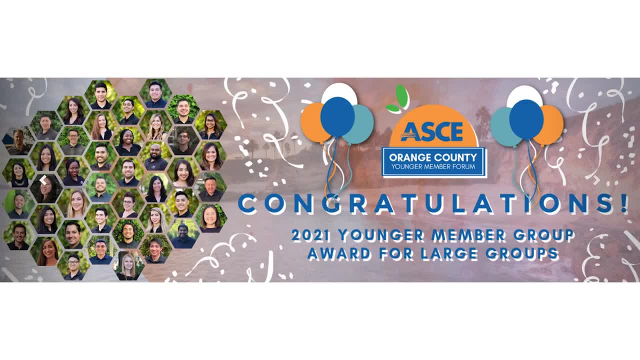 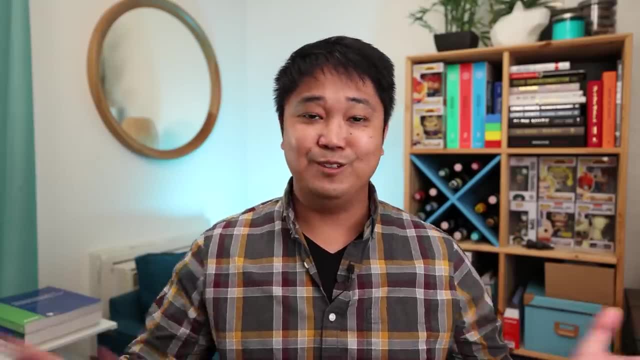 I joined professional organizations such as ASCE, started this YouTube channel and became the structural engineering channel podcast host. I definitely went out of my comfort zone 20.. Lesson learned: If you think the industry should be better, if you think your company should be better, 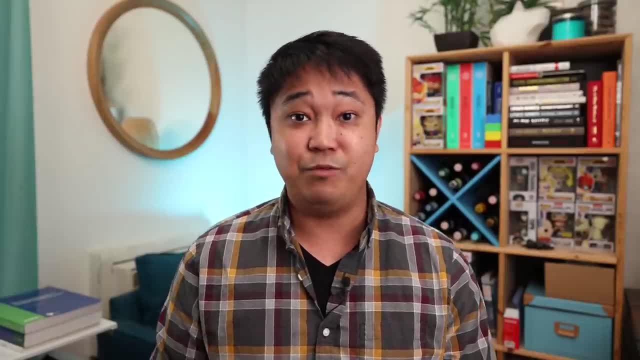 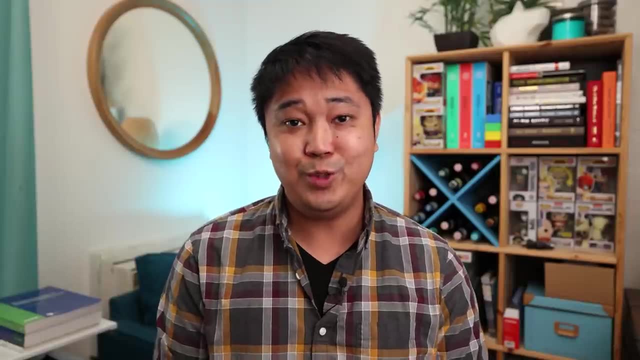 don't think somebody is going to do it, You're the person that's going to have to do it. Instead of saying, man, the structural engineering profession should get more exposure, you should do something about that. No one's going to do anything unless you do it first. 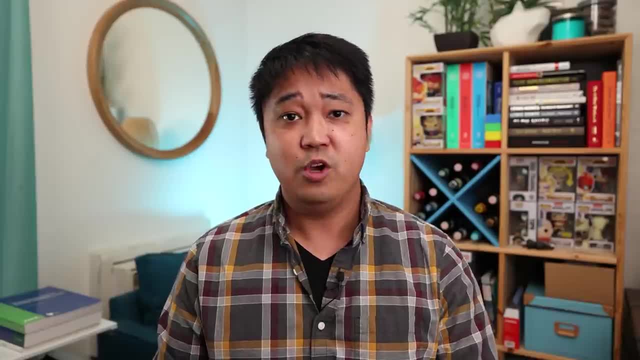 And as engineers, we may not be used to taking the lead on things or doing something that's really out of our comfort zone, like going on social media or whatnot. It was the exact same case with me. I didn't want to do anything. 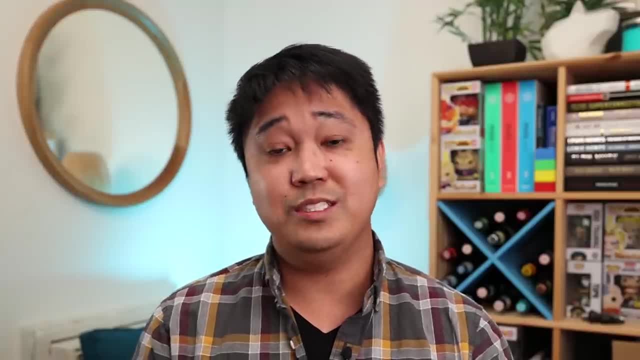 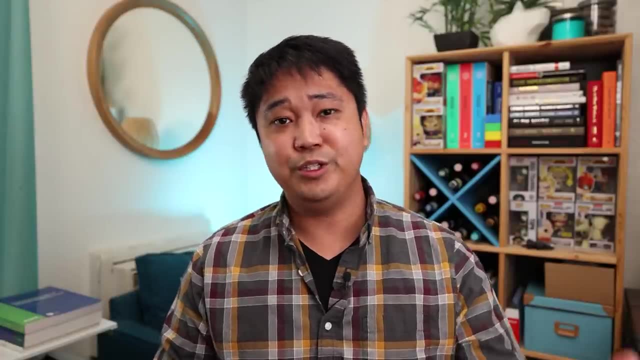 I didn't want to do any of these things. I didn't want to be on YouTube, but I knew YouTube was the way to go if I wanted to help a lot of engineers in their careers. You can do the same thing at work if you think your firm could do a better job of teaching. 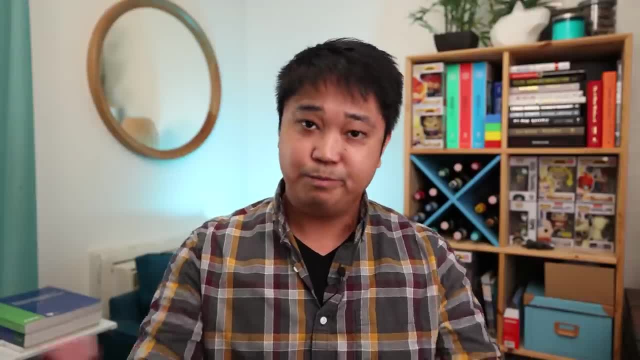 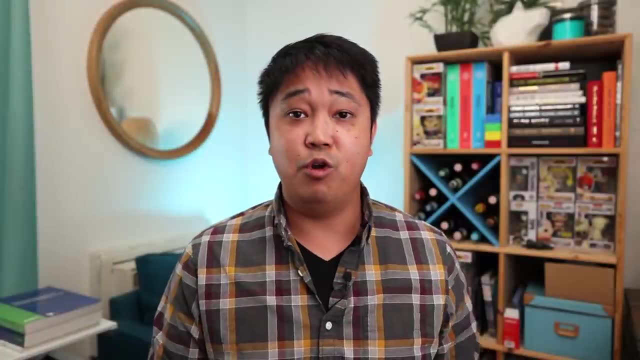 post-tension slabs, for example. Don't wait for someone to create the guide. You create the guide, you present it to your company and hopefully that can help your company out 20.. This was the year I started studying for my SC. licensing exam was heavily involved and 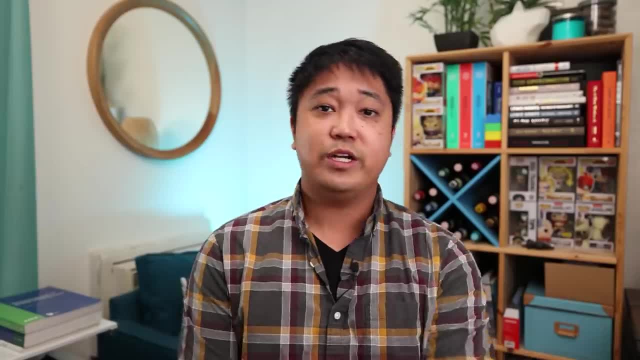 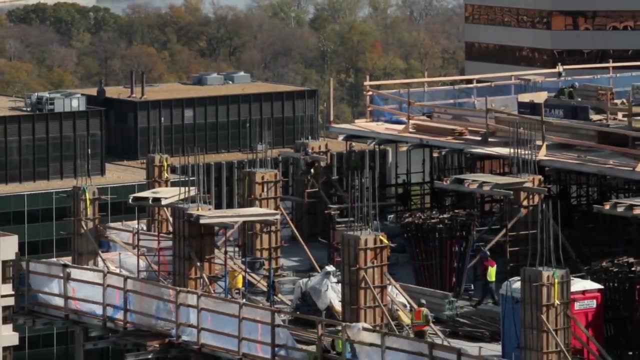 became an officer in my ASCE, YMF 20.. After work, I started to work on design-build projects like parking structures and tilt-up buildings. Design-builds were a lot more coordination and fast-paced than the typical project schedules that you're used to. 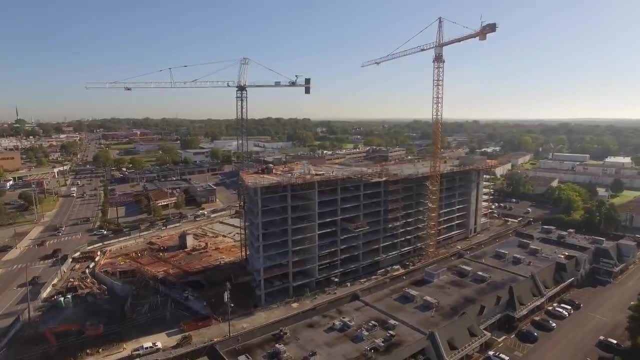 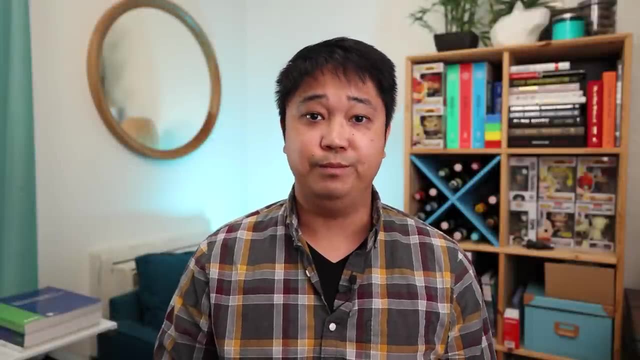 But I was starting to like them because they build it fast and the schedule's fast and you get to see the building get built in a year instead of two or three years. Lesson learned: Surround yourself with great people. They will lift you up when you're down. they'll guide you when you need help. you'll learn. 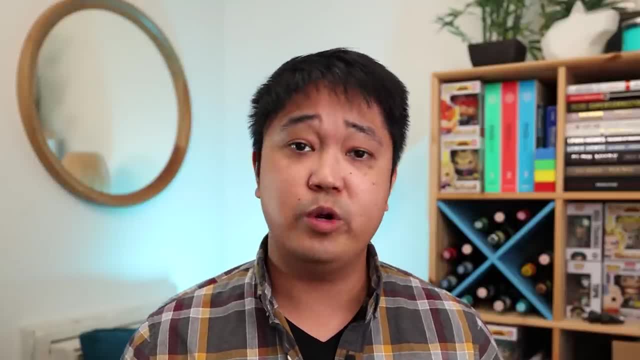 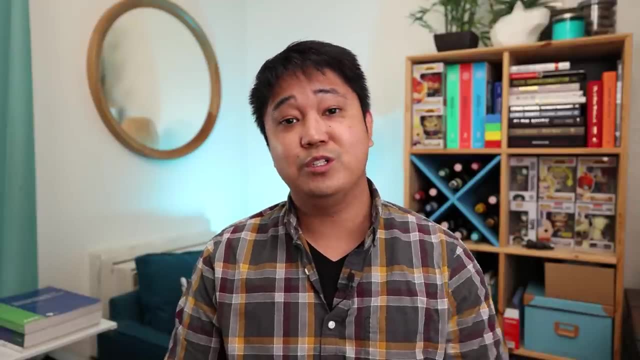 a lot from their leadership abilities and it'll open up a lot of career opportunities. 21. I learned just how important that was when I was working from home and failed my SC exam, From my coworkers, from my ASCE YMF group and from my friends and family.